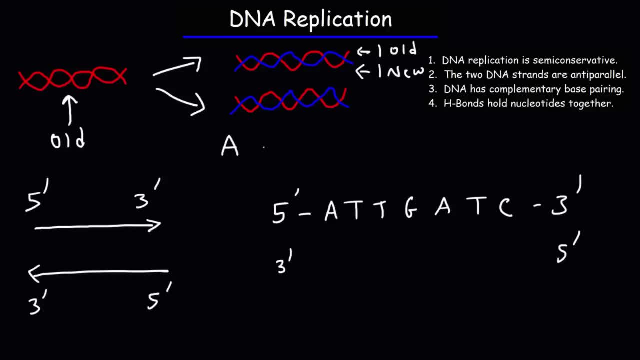 strand Now in DNA. you need to know that A always pair up with T and G always pair up with C and vice versa. So here we have A. A is going to pair up with T, T is going to pair up with A. 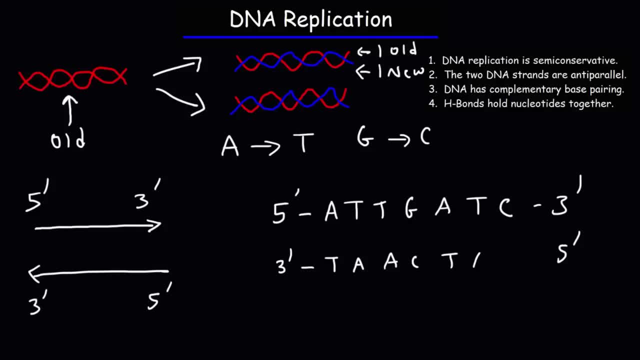 G is going to pair up with C, A is going to pair up with T, G is going to pair up with T and C will pair up with G. So, given the information of one strand, we can write the nucleotide sequence of another strand, And so that's the idea of complementary. 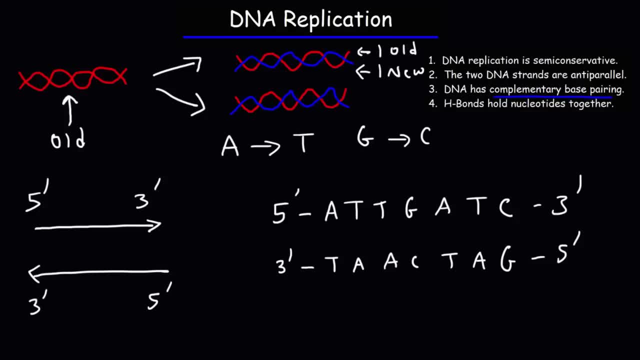 base parent in DNA. Now the next thing you need to know are what holds nucleotides together, And the answer is hydrogen bonds. Between adenine and thymine, there are two hydrogen bonds, And you need to know that between 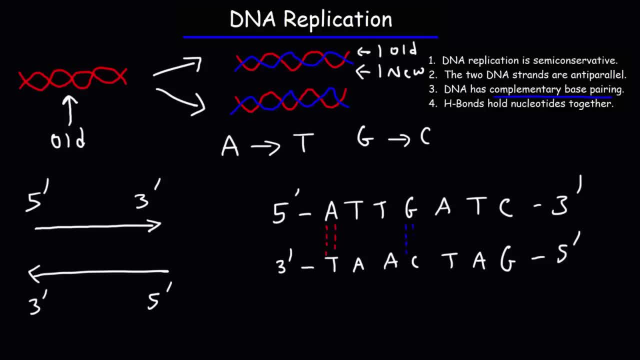 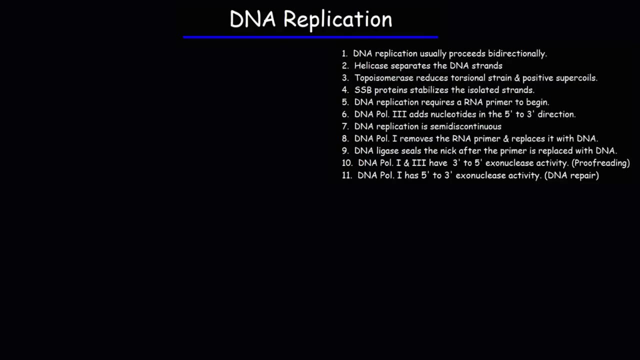 guanine and cytosine. there are three hydrogen bonds holding them together, So those H bonds are holding the DNA strands together. Now, there's a lot of other stuff that we need to talk about, one of which is that DNA replication usually proceeds bidirectionally. So what does that mean? Well, let me draw a. 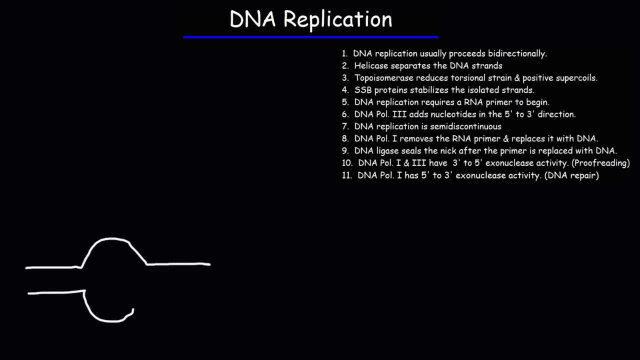 picture that will illustrate this concept. So this bubble that you see between the two strands, that is the origin of replication. In red, this is a new strand being produced Now in bidirectional DNA replication the strands can be produced in both directions, by means too, Now another. 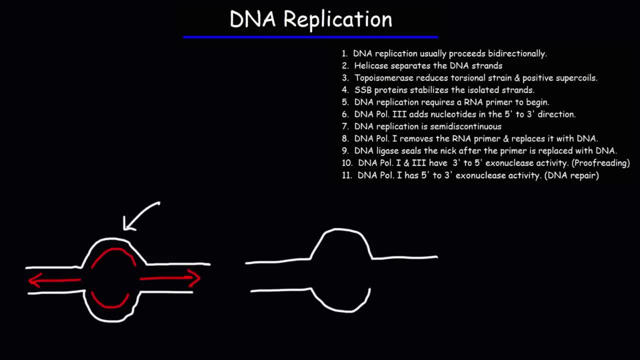 example of replication is unidirectional replication, So that occurs when the strand is being synthesized in one direction. So here's a picture of the replication fork that I decided to draw ahead of time, And the first thing that we're going to talk about is the helicase enzyme. Helicase separates the two strands. 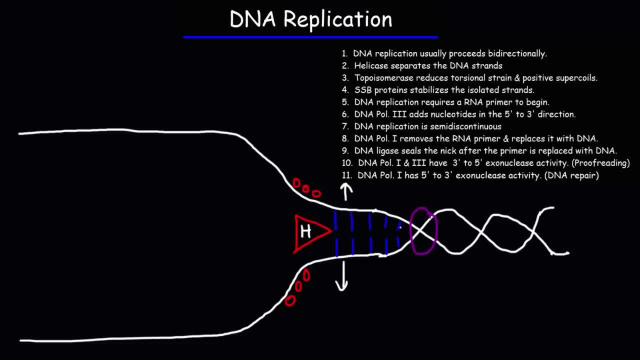 and it does so by breaking the hydrogen bonds that hold the nucleotides together. As helicase separates the two strands, torsional strain is created ahead of the replication fork And, as a result, an enzyme is needed, DNA gyrase, which is a type of topoisomerase. And these types of 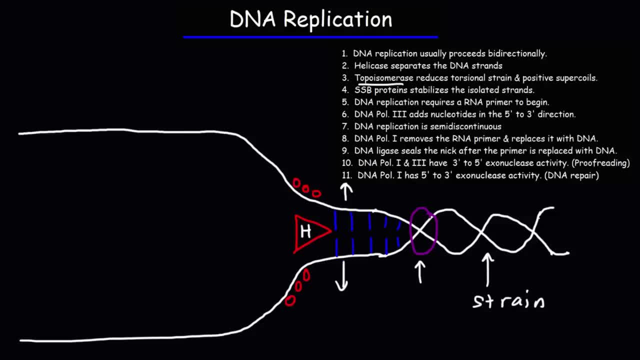 enzymes. they can reduce the torsional strain and even the nucleotides. So here's a picture of a positive supercoilin that could form in the DNA strand ahead of the replication fork. So I'm going to put T for a topoisomerase enzyme, So you might see DNA gyrase here as well. but keep in mind that 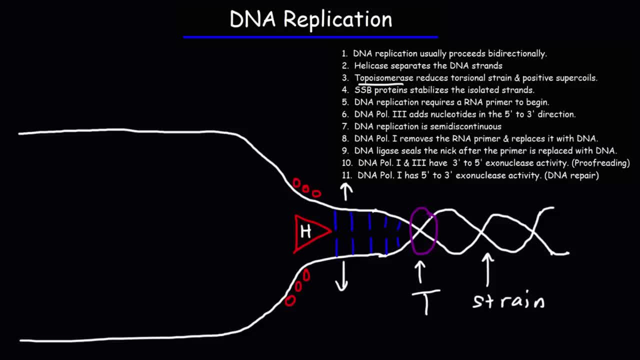 DNA gyrase is a type of topoisomerase enzyme. Next we have the SSB proteins, the single stranded binding proteins. These SSB proteins: they protect the two strands from cleavage. they also stabilize the two strands, preventing them from snapping back together. Now DNA. 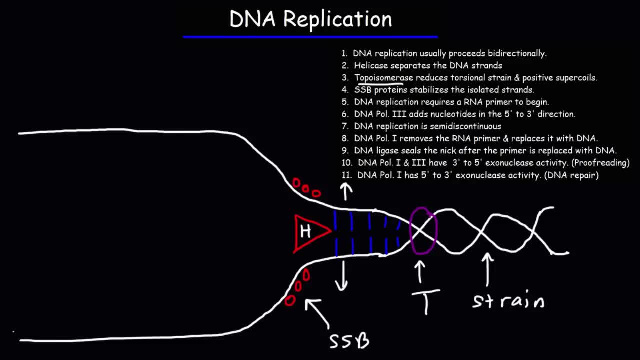 replication requires an RNA primer to begin, So I'm going to draw the RNA primer in green. The RNA primer is basically a sequence of RNA nucleotides. DNA polymerase III: once it sees the RNA primer, it begins to produce a sequence of RNA nucleotides. So it's a sequence of RNA nucleotides. So it's a. 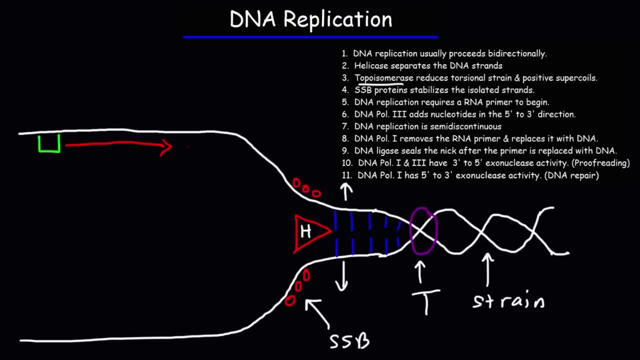 to synthesize the new strand in the 5 to 3 direction. This strand here is called the template strand And that strand runs in the 3 to 5 direction. But DNA- I mean DNA polymerase 3, is going to build the new strand in the 5 to 3 direction. 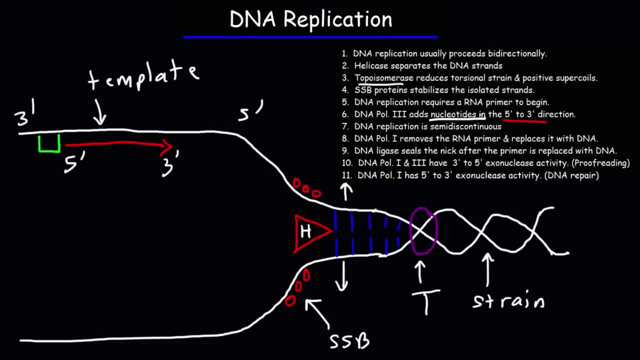 So make sure you understand that DNA polymerase 3 adds nucleotides in the 5 to 3 direction. Now the enzyme that creates the primer is known as primase. Now, DNA replication is semi-discontinuous. Now what does that mean? 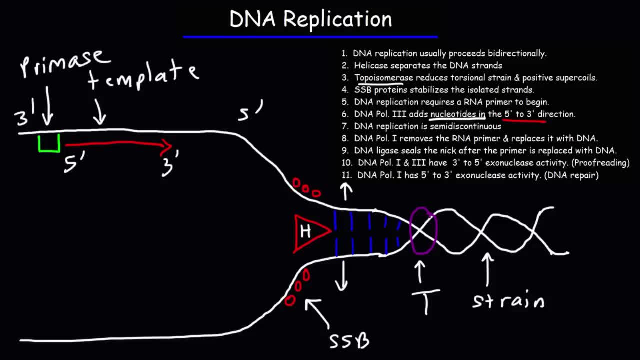 What does it mean that DNA replication is semi-discontinuous? Well, we need to talk about the other strand. So the first template strand on top runs in a 3 to 5 direction, which means the template strand on the top runs in a 3 to 5 direction. 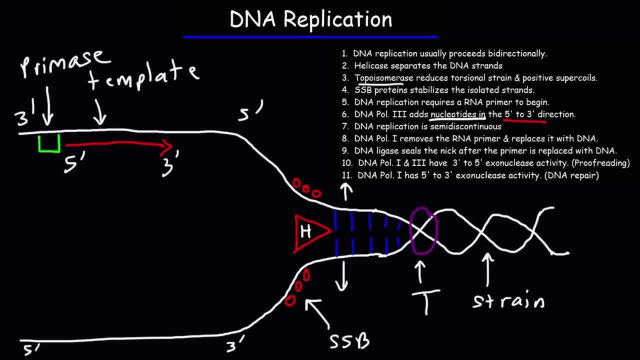 And the second template strand on the bottom runs in the 5 to 3 direction. DNA polymerase 3 only adds nucleotides in the 5 to 3 direction. So once a primer is added to this strand, DNA polymerase 3 is going to work in this direction. 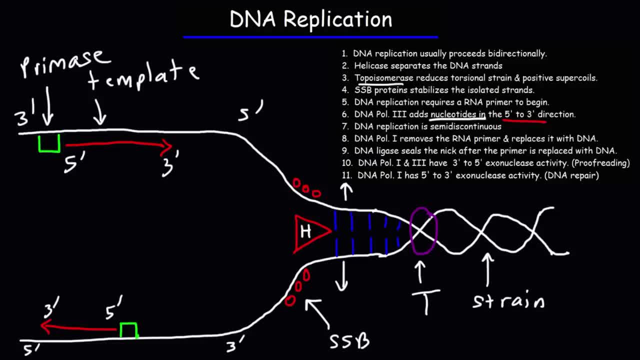 That is, in the 5 to 3 direction. Now notice that this strand- this strand, by the way, is called the one in red- this is called the leading strand And this one here is called the lagging strand. 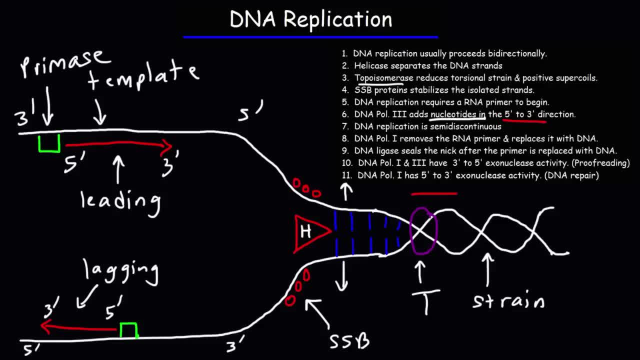 The leading strand moves in the same direction as the replication fork. The lagging strand moves in the opposite direction of the replication fork. So as the replication fork continues to move forward, you're going to have a lot of trouble. You're going to have more space here. 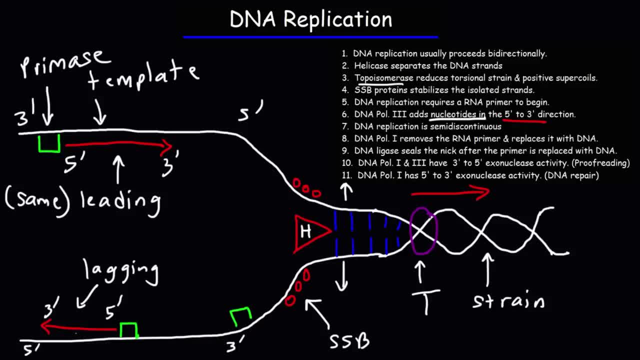 So what's going to happen is a new RNA primer is going to join here and then DNA polymerase is going to start there, producing or adding nucleotides in this direction. So in the leading strand, DNA is synthesized continuously. It only needs one primer to start. 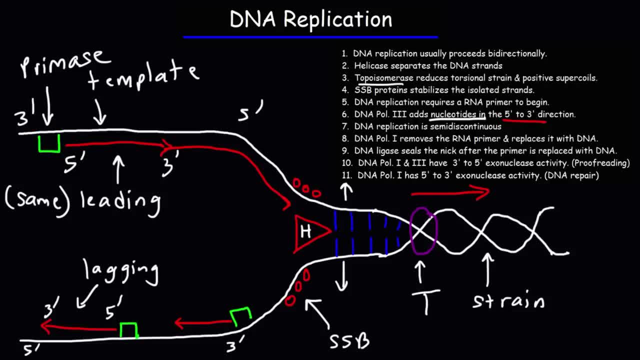 and it just keeps on going. It follows the replication fork On the lagging strand. it doesn't synthesize a new strand continuously. The replication is discontinuous, As you can see here with that empty space. So that's why DNA replication is said to be semi-discontinuous. 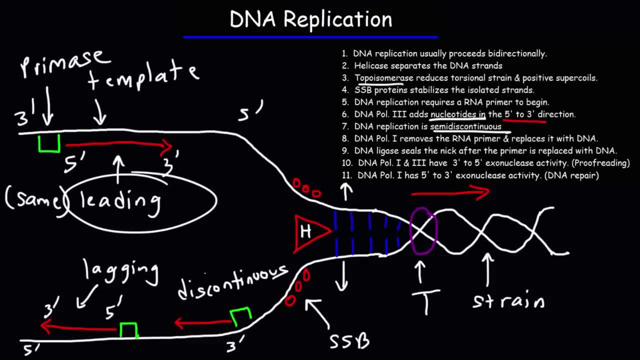 It's continuous in the leading strand but discontinuous in the lagging strand. The prefix semi- means half, So it's half continuous, half discontinuous. So technically you could say semi-discontinuous or semi-continuous. Both words will accurately represent DNA replication. 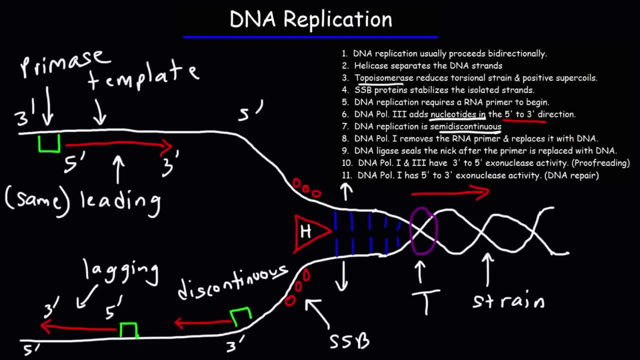 Now DNA polymerase 1 removes the RNA primer and replaces it with DNA. So after replication, when it's almost finished, this part, this RNA primer gets replaced and it's removed, And so I'm going to replace that with a red color. 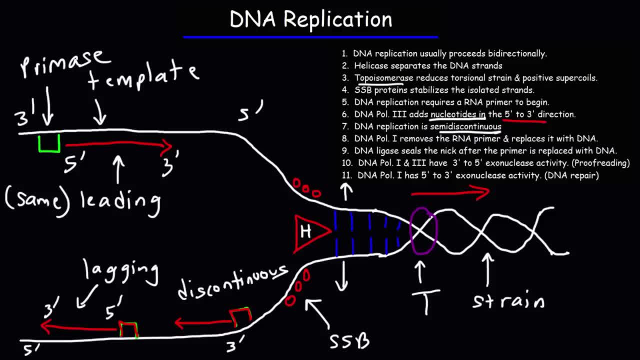 So it's been replaced by DNA polymerase 1.. Well, I mean, DNA polymerase 1 replaces the RNA primer with DNA material. Now, once that happens, you're going to have some spaces in between. By the way, these fragments are called. 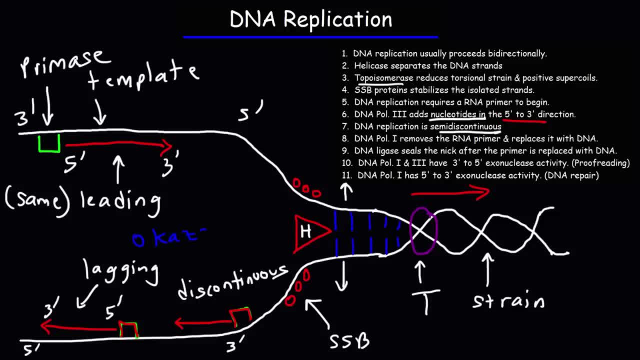 Okazaki fragments, Okazaki fragments. Hopefully I spelled that correctly. Now another enzyme called DNA ligase seals the nick between the Okazaki fragments, And so there you have DNA replication. So that's the whole process. there Now some of the things. 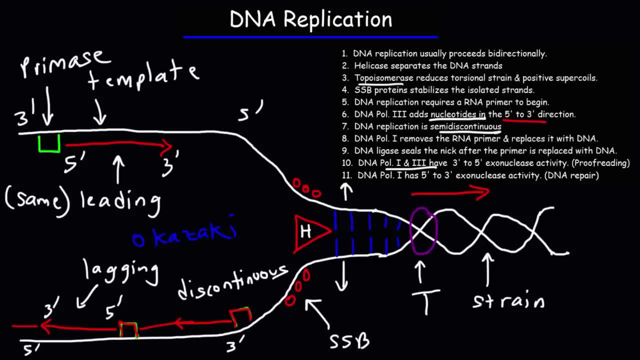 that you want to know is that DNA polymerase 1 and 3, they have 3 to 5 exonucleases activity. An exonuclease enzyme is an enzyme that can remove nucleotides from a strand, starting at one end of the strand. 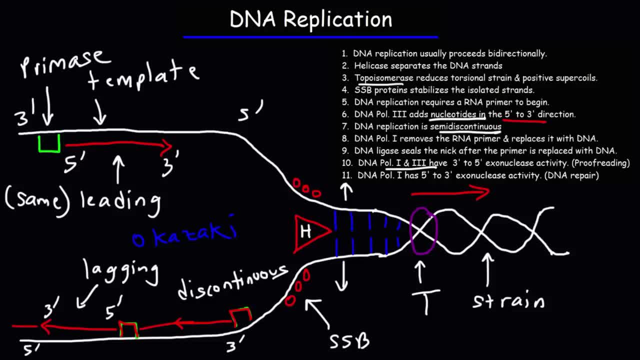 So this 3 to 5 exonuclease activity? it describes the proofreading ability of these two enzymes. So when DNA polymerase 3 is synthesizing a new strand, if it makes a mistake it can stop, remove the wrong nucleotide. 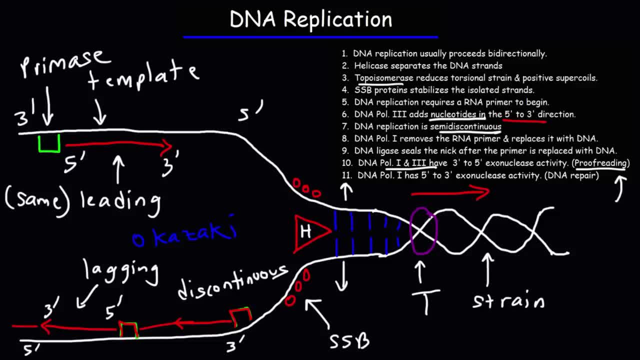 and replace it with the right one. So that would be the proofreading ability of DNA polymerase 3.. Now, DNA polymerase 1, not 3, has the 5 to 3 exonuclease activity which plays a role in DNA repair. 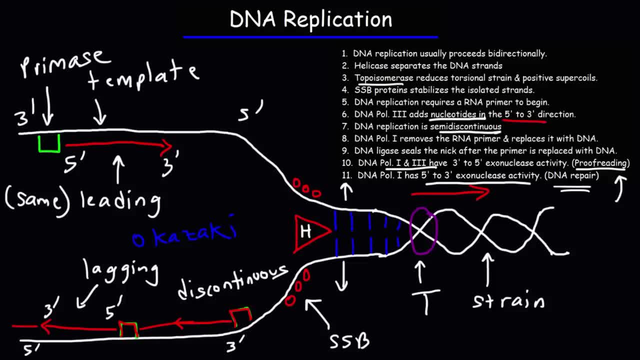 So those are some things that you want to know with regard to DNA replication. So just to review, DNA ligase is the enzyme that seals the nicks between Okazaki fragments, and then DNA polymerase 1, is the enzyme that removes. 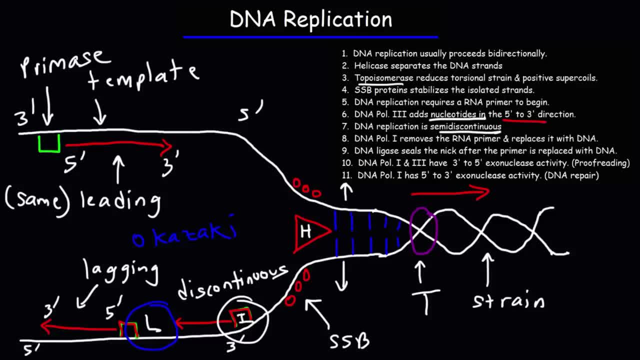 the RNA primer and replaces it with DNA material prior to ligase, sealing the nicks. And then also DNA polymerase 3 is the enzyme that builds the new DNA strand during elongation. So make sure you understand the functions of those enzymes. 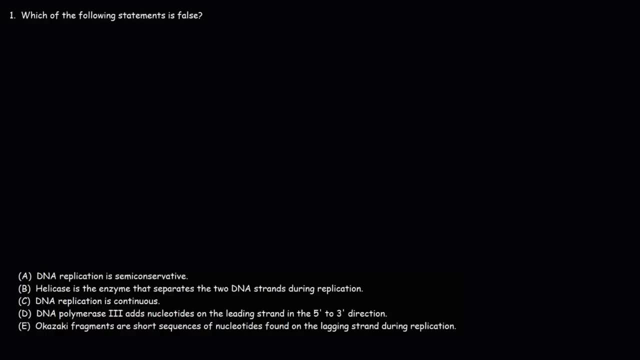 And so that's basically it for DNA replication. Now let's work on some practice problems. for the sake of review, Feel free to pause the video if you want to try this mini quiz. Number one. which of the following statements is false? So let's look at A. 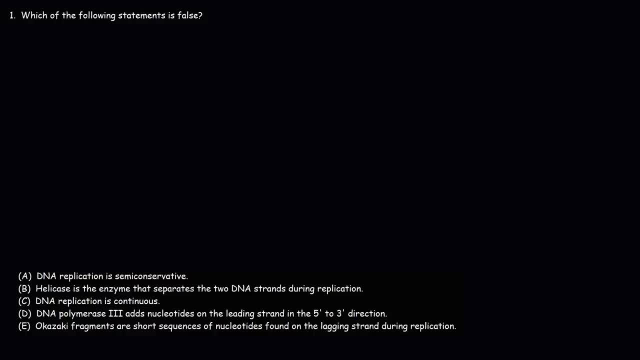 DNA replication is semi-conservative, Would you say that's a true statement or a false statement? Now, that statement is true: DNA replication is semi-conservative. If you recall, we start with an old DNA strand And once we create two copies. 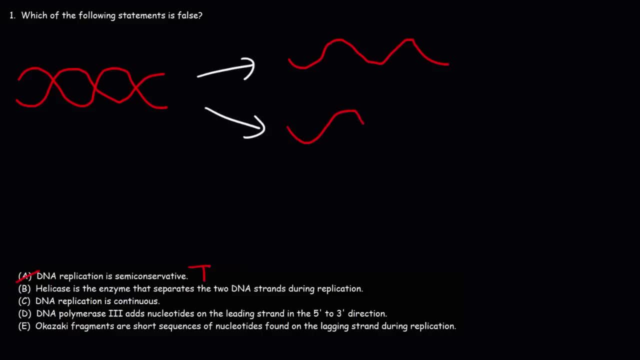 each copy will have one old DNA strand And each copy will have one new DNA strand. So it's semi-conservative in that each new copy has one old strand and one new strand. Some other ideas of DNA replication are conservative and dispersive replication. 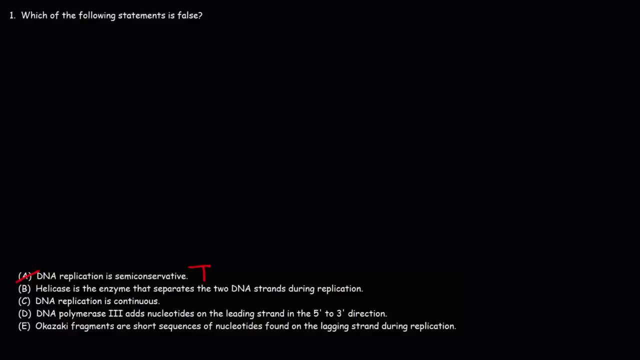 Now B. helicase is the enzyme that separates the two DNA strands during replication. Is that true or false? So that is also a true statement. Helicase is the enzyme that breaks the hydrogen bonds between the nucleotides that are holding the two strands together. 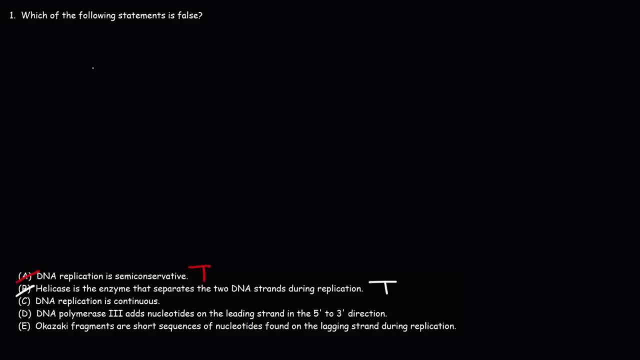 And that's how it separates them during replication. Here is a visual illustration of that. So here are the hydrogen bonds that are holding the two strands together, And here is helicase, which is about to break those hydrogen bonds. This is going to open the DNA strand. 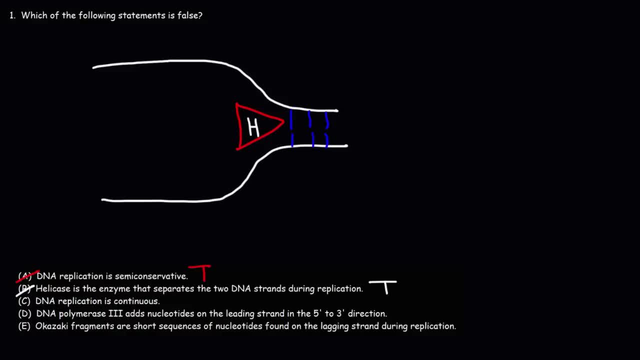 and separate into two parts. Now, DNA replication is continuous. Is that true or false? So this is a false statement. DNA replication is semi-discontinuous, or you could say semi-continuous The leading strand, which is the DNA strand. 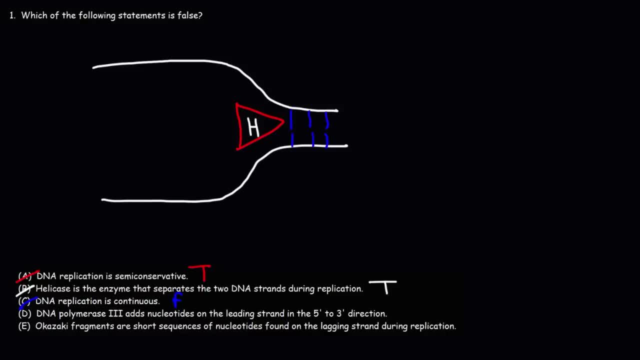 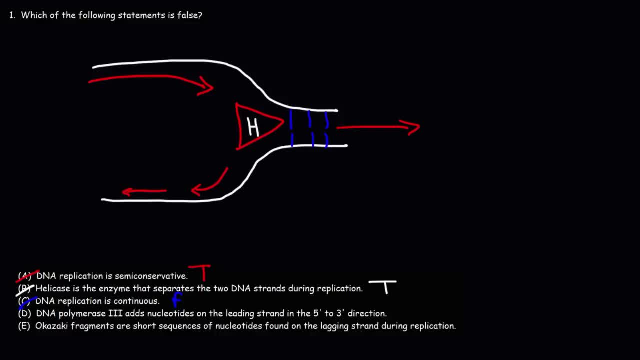 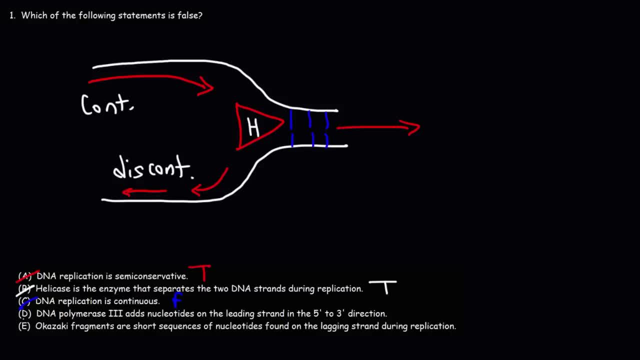 DNA replication is semi-discontinuous. DNA replication is semi-discontinuous. DNA replication is semi-discontinuous. Enapolymerase III adds nucleotides on the leading strand in the 5 to 3 direction, And E Okazaki fragments are short sequences of nucleotides found on the lagging strand during replication. 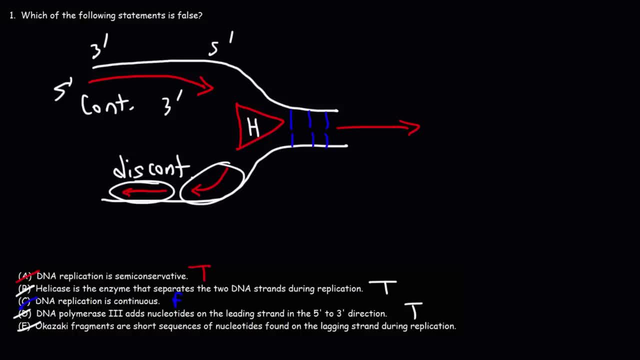 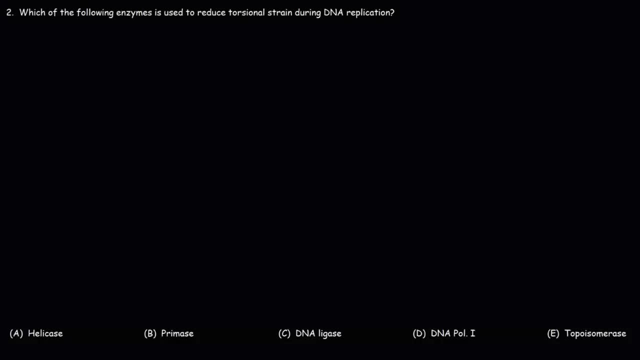 So these would be the Okazaki fragments. So the answer for this problem is C. That is the false statement Number 2.. Which of the following enzymes is used to reduce torsional strain during DNA replication? Is it Helicase Primase, DNA Ligase, DNA Polymerase I or Topoisomerase? 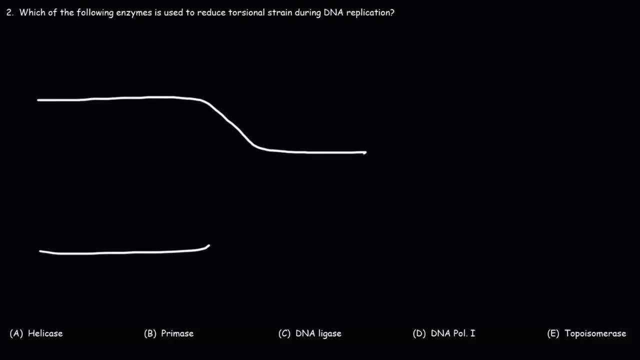 What would you say? So feel free to pause the video to work on it, So we know. the answer is not A. As we said before, Helicase is the enzyme that breaks the hydrogen bonds, thus separating the two strands. So A is out. 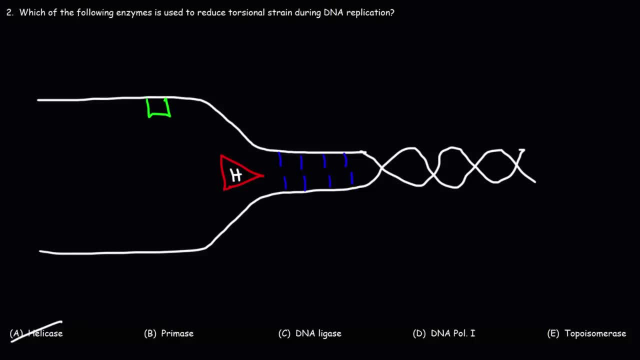 Primase is the enzyme that synthesizes the RNA primer representing green. Ligase is the enzyme that seals the nicks that are formed in between the Okazaki fragments, So Ligase will be here. DNA Polymerase I is the enzyme that removes the RNA primer and replaces it with DNA material. 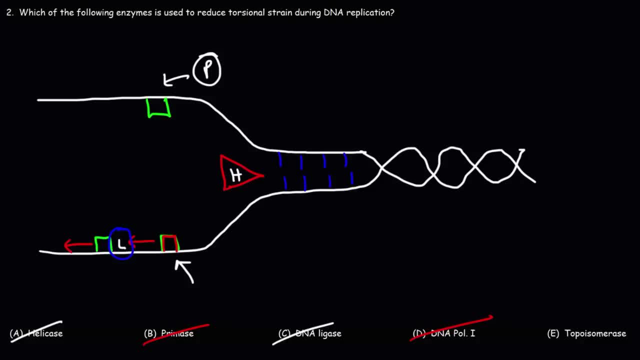 So E is the correct answer? The answer is E. The Topoisomerase enzyme is the enzyme that relieves the torsional strain that is built up when Helicase separates the two strands. So E is the correct answer, Number 3.. 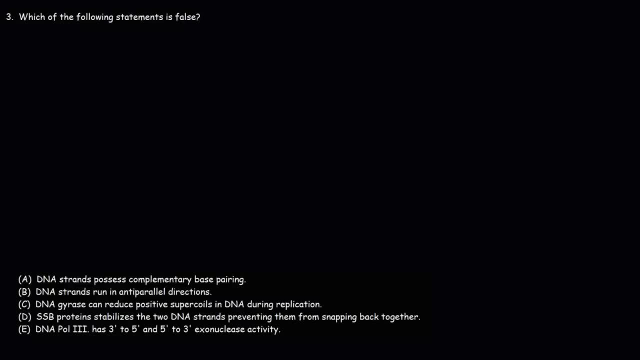 Which of the following statements is used to reduce the torsional strain? false, So let's go through each one, one at a time. Looking at answer choice: A DNA strands possess complementary base pairing. Is that true or false? This is a true statement. So if the first strand 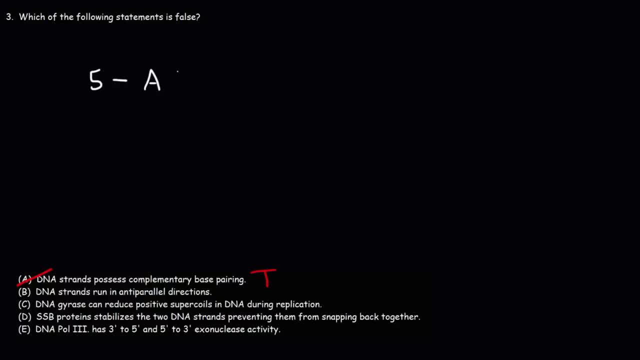 has, let's say, the nucleotide sequence A, G, T, T, G, C, A, T, G. What's going to be the nucleotide sequence of the other strand? It's going to run in the other direction. A always pairs up with T. 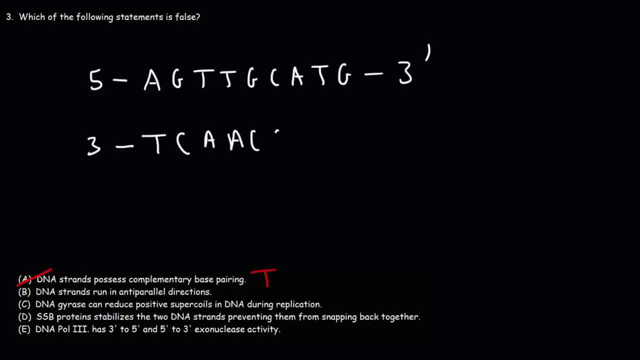 C always pairs up with G, So we'll get this sequence, And so this is an example of complementary base pairing. And don't forget that there's two hydrogen bonds between adenine and thymine, and there's three hydrogen bonds between guanine and 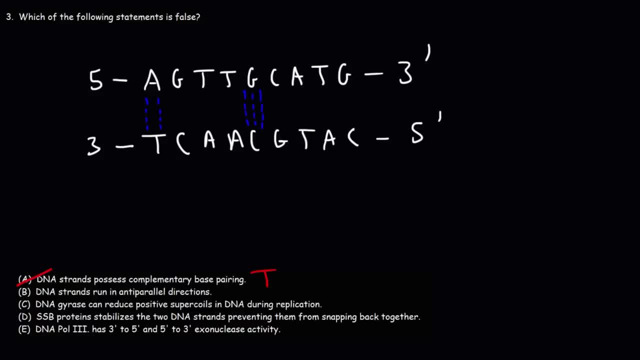 cytosine. Now B DNA strands run in anti-parallel directions. That's a true statement. If one strand goes in the five to three direction, the other strand is going to run in the opposite direction. So they're anti-parallel. Now looking at part C, 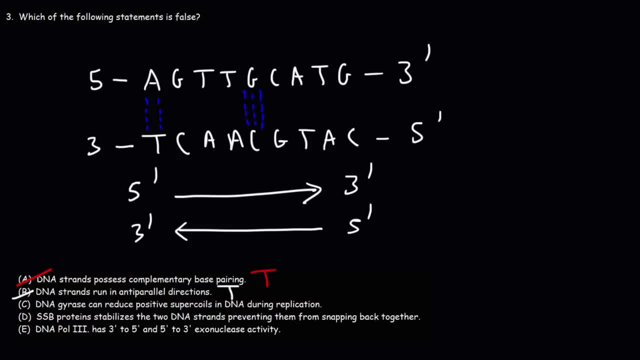 DNA strands run in the opposite direction, So they're anti-parallel. DNA strands run in the opposite direction, So they're anti-parallel. Now looking at part C: DNA gyrase can reduce positive supercoils in DNA replication. That's also a true statement. 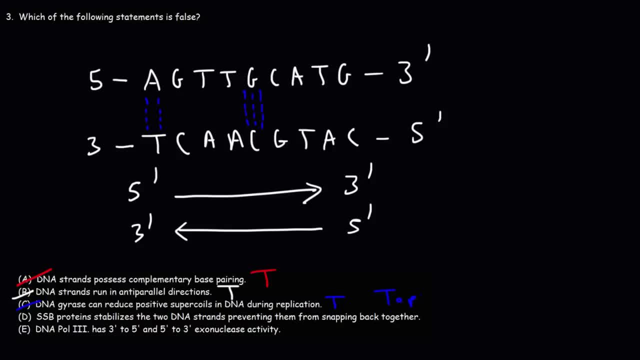 Keep in mind, DNA gyrase falls in the category of topoisomerases. I always have issues saying that word. So DNA gyrase, a type of topoisomerase, can reduce positive supercoils and can reduce torsional strain ahead of the replication fork. So DNA gyrase can reduce positive supercoils and can reduce torsional strain ahead of the replication fork. So DNA gyrase can reduce positive supercoils and can reduce torsional strain ahead of the replication fork. So DNA gyrase can reduce positive supercoils and can reduce torsional strain ahead of the replication fork. 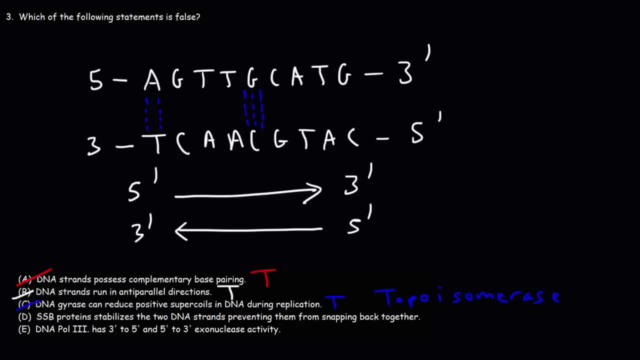 DNA replication. Sometimes my words just don't flow smoothly off my tongue. What can I say? it just happens. Now let's move on to part D: SSB proteins, or single-stranded binding proteins, stabilizes the two DNA strands.